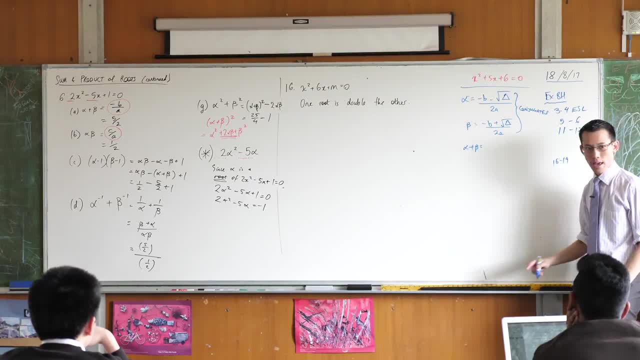 Watch, Let's have a look. You can write this with me, because it's that simple, right Alpha plus B, Beta, Because you're adding these things together. what happens bless you to this square root part. What happens? 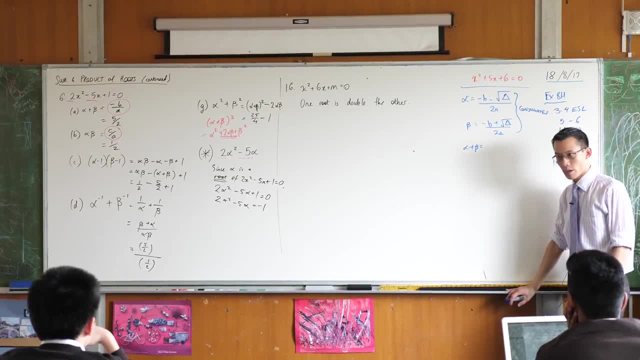 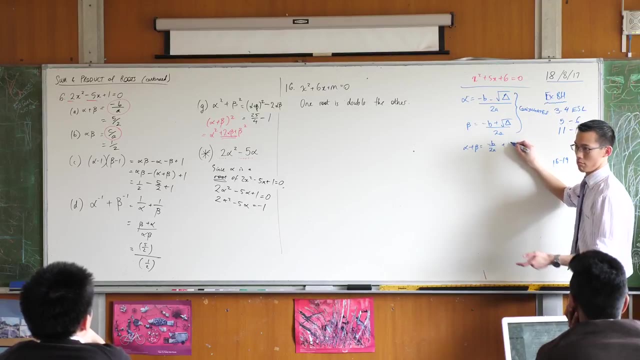 When you add these two things together, they're going to cancel out. This is just like solving a set of simultaneous equations by elimination, isn't it? These things are going to eliminate, So all you get left with is minus B on 2A plus minus B on 2A. 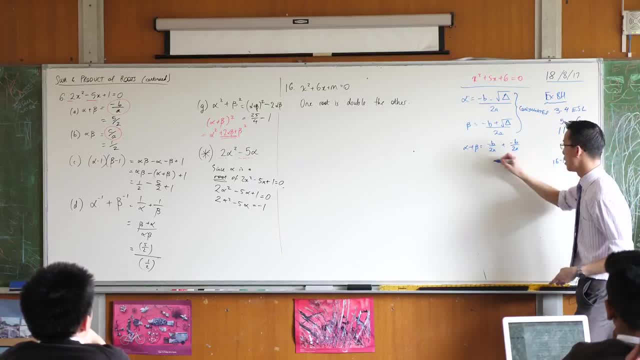 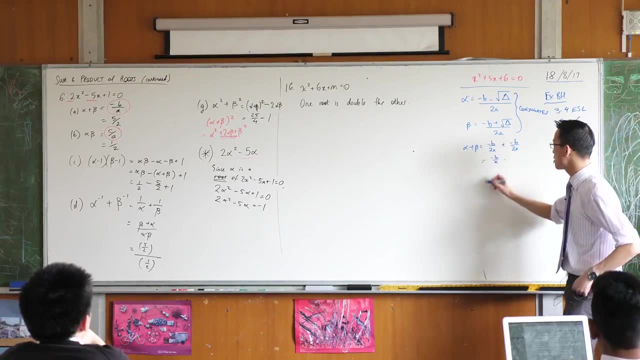 The square root of the discriminant. It's both gone. They've cancelled each other out. Well, this is clearly. look what happens, right? Well, this is minus B on A. Do you agree? The same thing happens when you do the product. 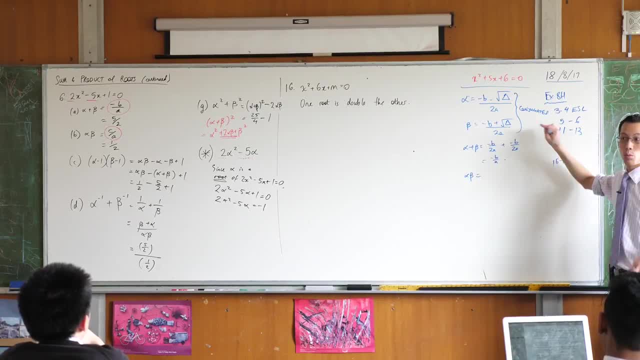 It looks like it's going to be disastrous, but remember they are conjugates, So we should have some faith that this is going to come out nicely in the wash right. This is going to be this guy and this guy on the top. 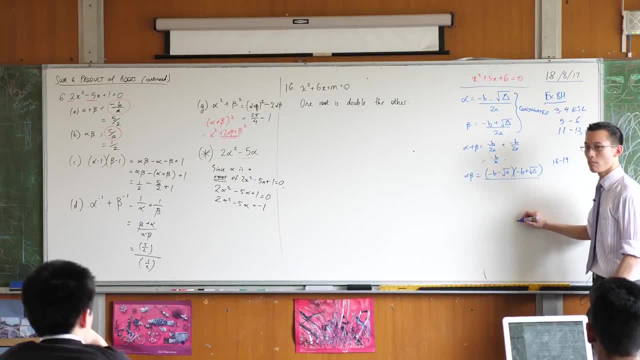 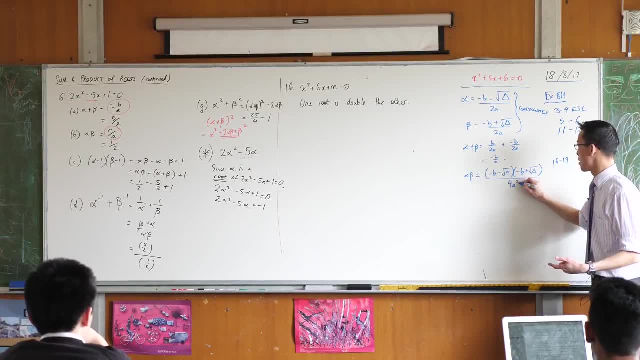 Four, Four, Four, Four, Four, Four, Four, Because 2A times 2A. Now again, this looks terrible, but hold on, they're conjugates. So what happens to these guys? What is this? 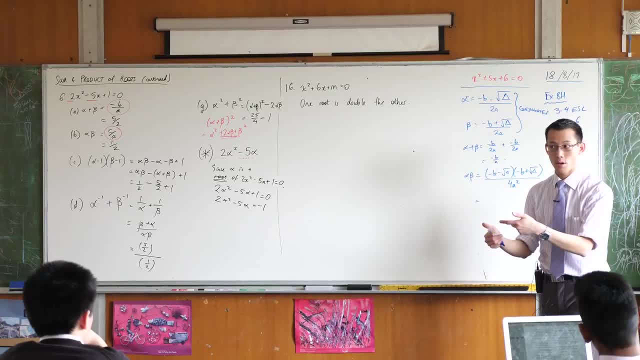 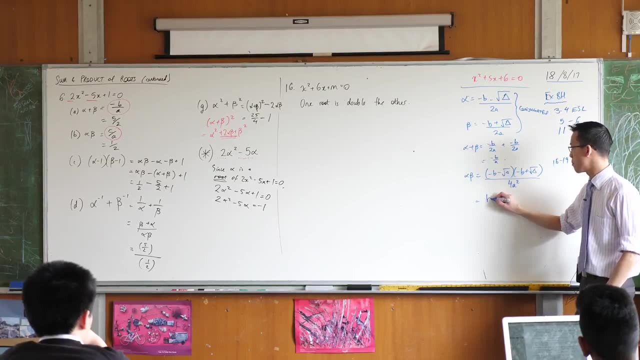 What is this? a factorization of? This is difference of squares, isn't it? So what's the first thing, What's the first square? It'll be B squared. right, That's the square of this thing here. Then I'm going to take away this squared. 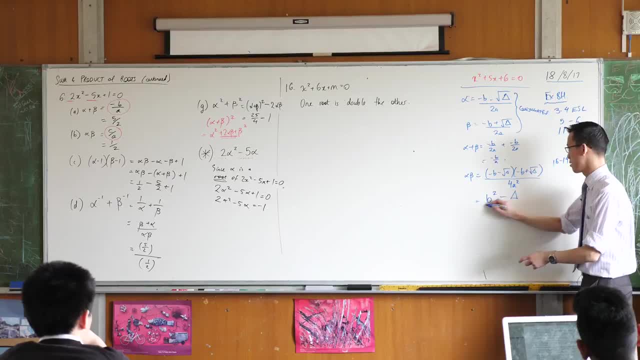 Yeah, Which is just this. on this, Are you with me so far, But you know what the discriminant is, don't you? The discriminant is B squared minus 4AC. Just watch out, bud. There's a negative there. 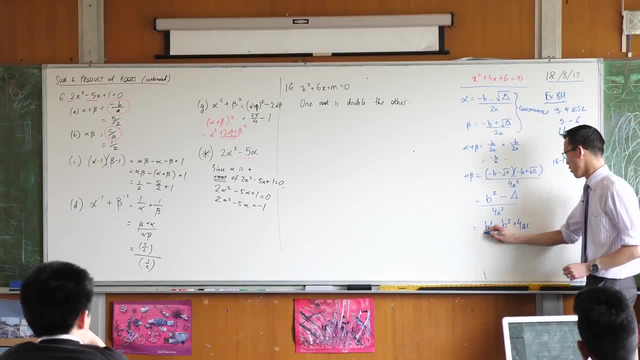 So this is actually a double negative. Are you okay with that? You see how I'm just Yep, All over 4A squared. Well, this is just cancel city, isn't it Watch? Cancel, Cancel, Cancel, Cancel. 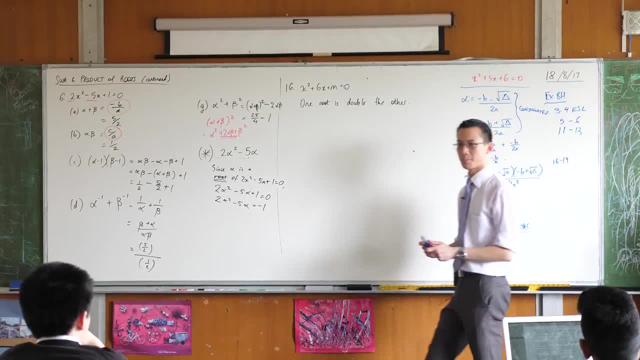 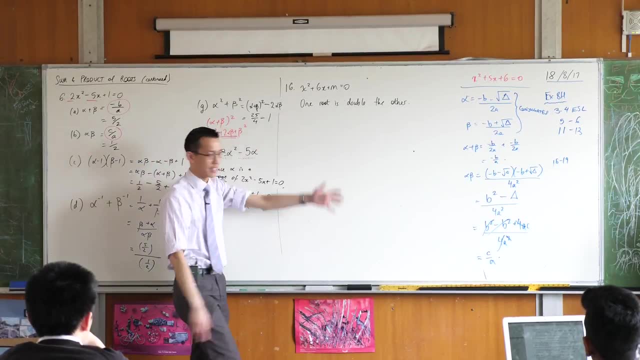 There's your C on A, just like we proved this morning. Okay, So if you have a trouble remembering which one is, which it actually doesn't even take that much thought. I just wanted to show you. it's another way of getting to the same thing and really as 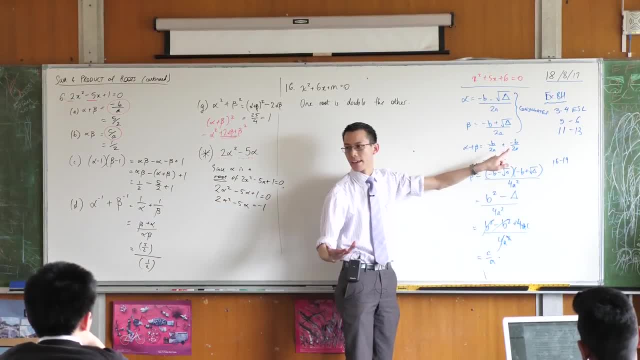 soon as you get to this line here, when you're like, oh, I'm adding these things and they're both negative, well, clearly that gives you the negative one. Does that make sense? I'm not sure. Say it again, I'm not sure. 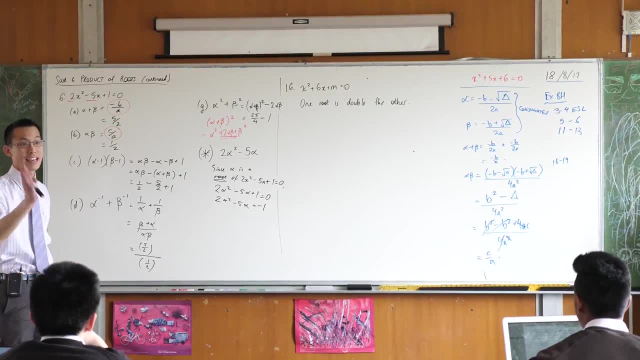 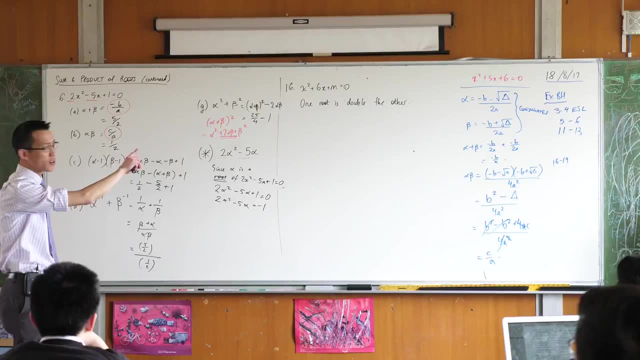 Correct, But I want you to know them. You shouldn't need to look at them. You shouldn't need to take that time to look at it for that, Okay. last example: I wanted to have you, i wanted to have a go. i don't think anyone's up to this, are they? no, okay, except for jason, okay. 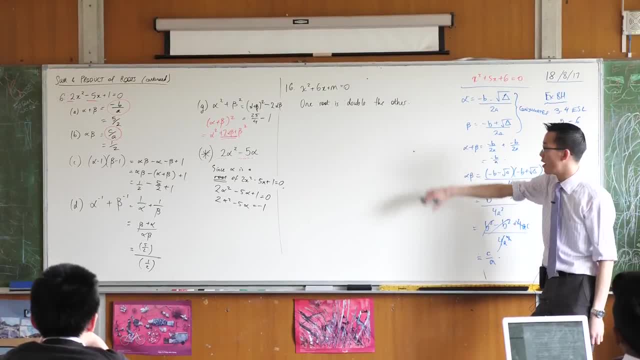 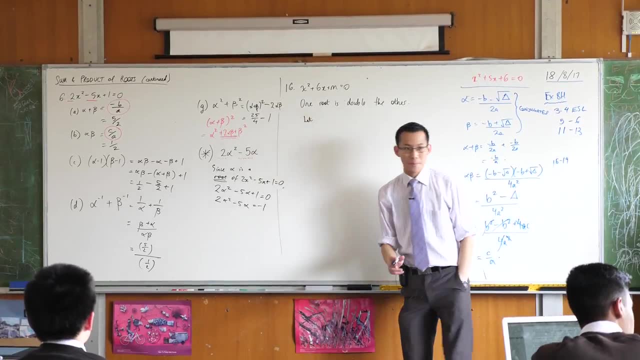 good on him. that's fine. let's quickly have a go at this so everyone can write this down. this is question 16, so it's buried a little bit toward the end of the exercise, but it's easy enough to do. okay, now, in all of these contexts i've sort of just been assuming let's just call. 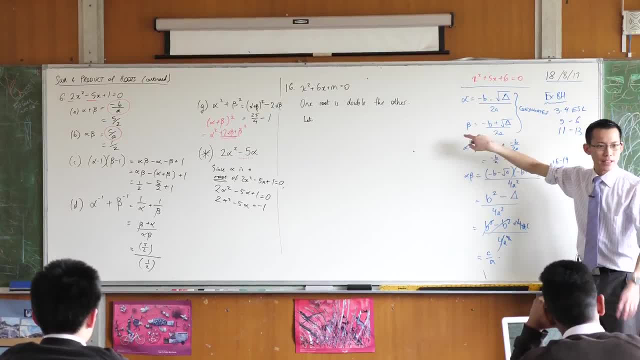 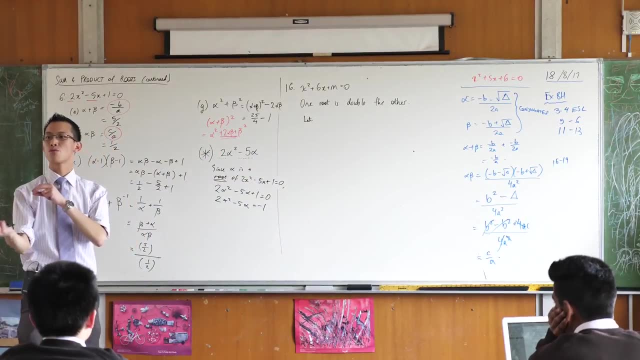 a root alpha and a root beta. okay, i don't know anything about them and so i just sort of define them independently. but often you get given information where you know one root is related to the other one, so you don't have to just give them random letters. you can say i don't need so. 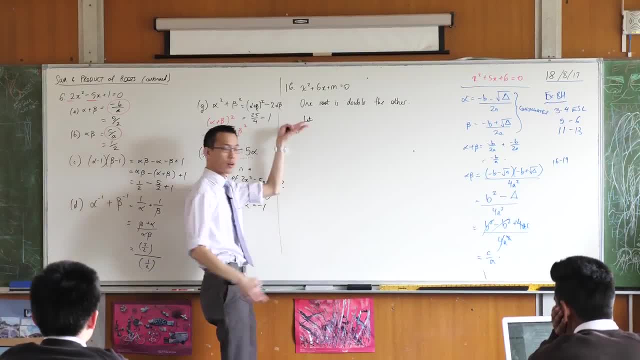 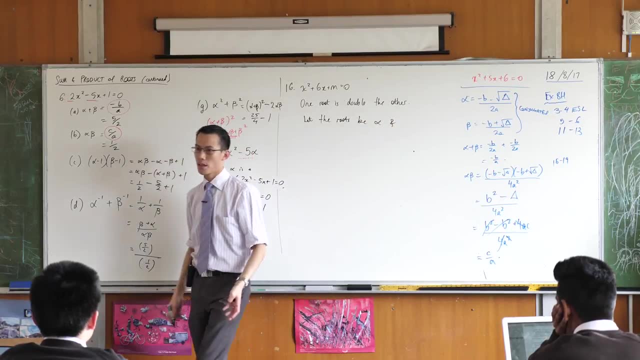 many protein rules, i can have them dependent on each other. so for this question i would say: let the roots be alpha. and now, instead of saying beta, i know that beta will be double the other one, so i'm just going to call it two alpha. just as equally, i could have called it alpha on two. 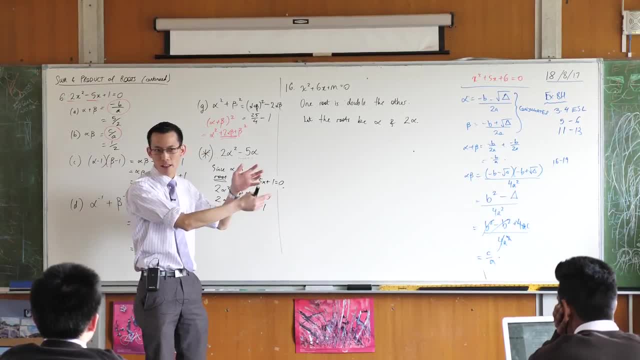 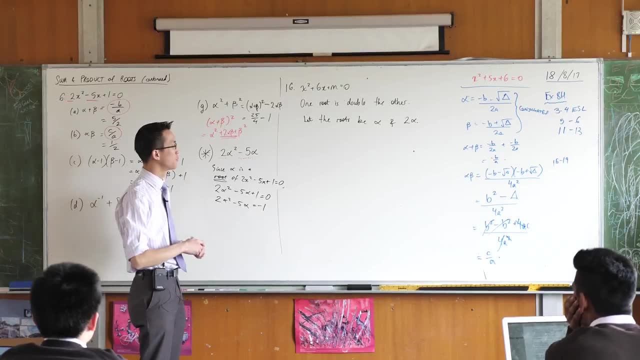 okay, okay, yeah, because one would still be double the other. why am i avoiding that? because i don't like fractions, so this is just fine. okay, sometimes you can't avoid fractions, but this time i will. so if the roots are alpha and two alpha, i can find the sum of roots just. 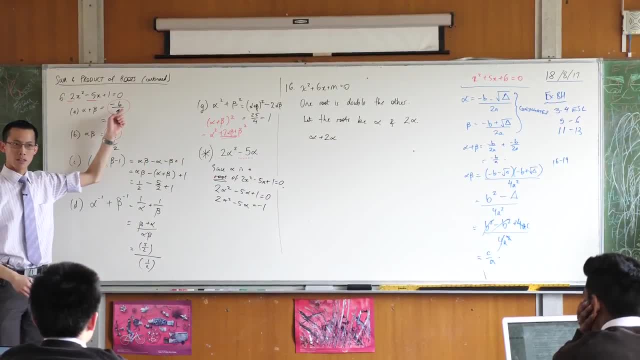 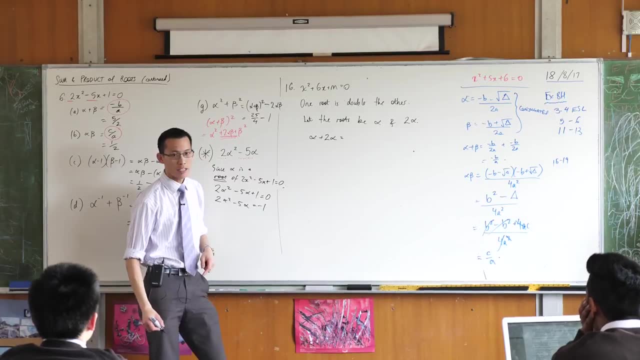 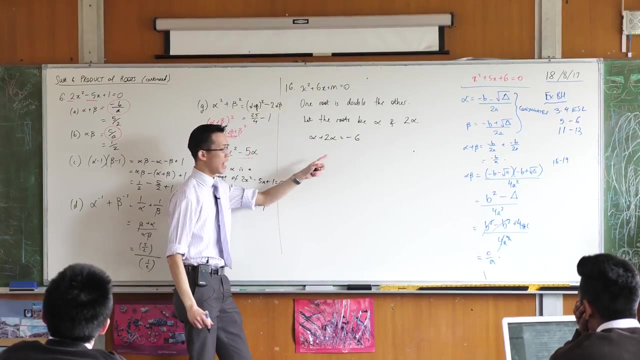 like i normally do with minus b on a. yeah, it's just, it's not alpha beta, it's alpha plus two alpha. so what's this? equal to minus b on a in this case is negative six, negative six, negative six. that's good, so you can see, here i can already work out what alpha is. that's nice, isn't it. 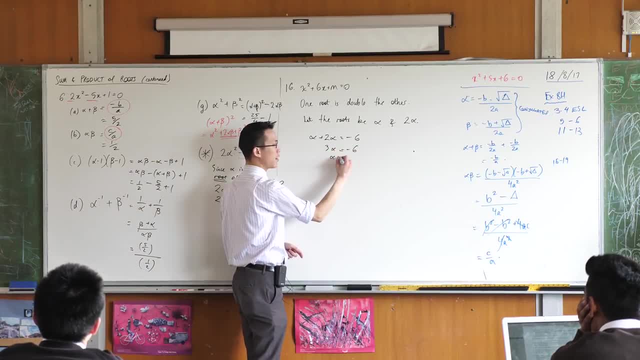 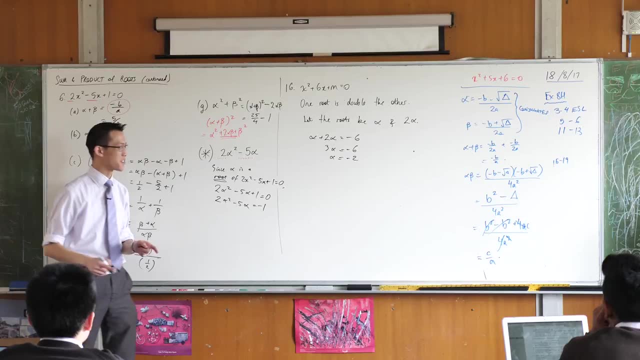 three alpha equals negative six, so alpha is equal to: okay, excuse me now, i didn't even tell you what the question was. didn't even tell you what the question was. we just started to launch into this, which is not that bad a strategy. you almost certainly have to do something with these. 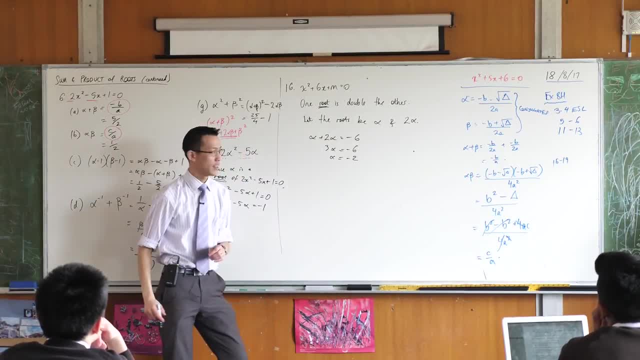 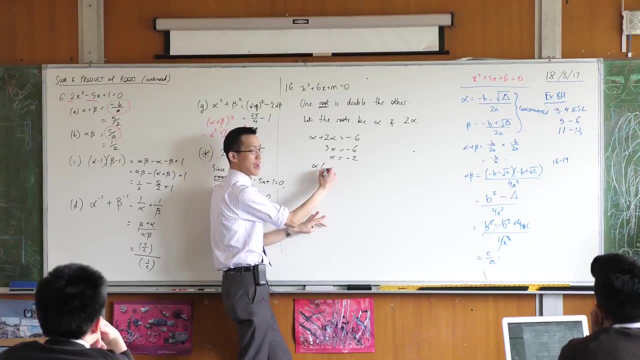 results if they say something like this: okay, but now you can see if i go to the next step. here's something that i'm going to do. i'm going to do something like this. i'm going to do something like this. i'm going to make a plus. some of roots, product of roots, will be alpha times two alphas. no, it's not. 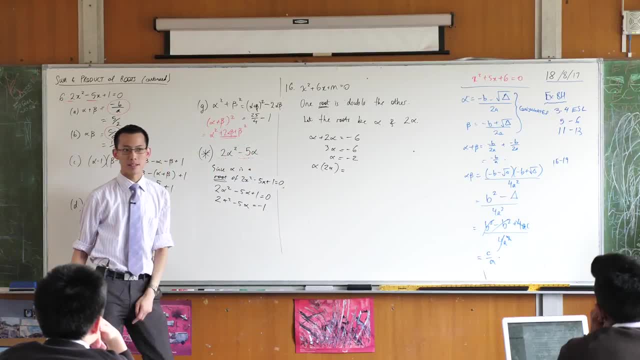 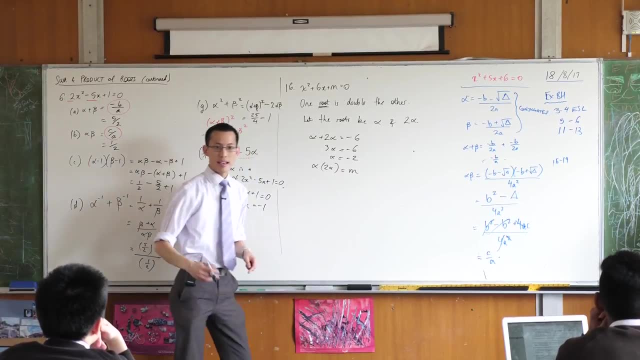 beta, is it? what is the number going to be? in this case, it's c on a, which in this case, is off, which always makes this for me. and as, so it happens, the question is asking us to find m, so we get over here to alpha square. 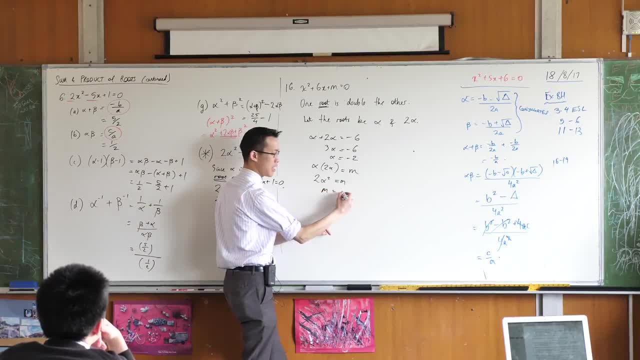 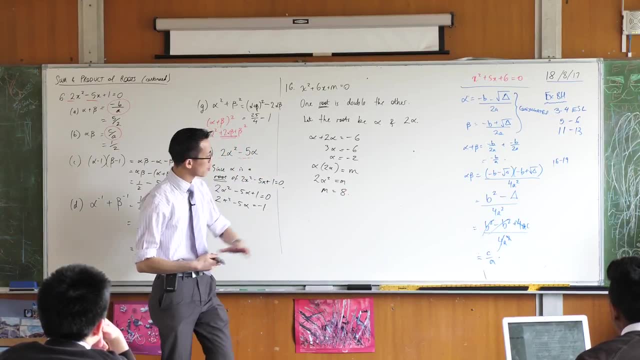 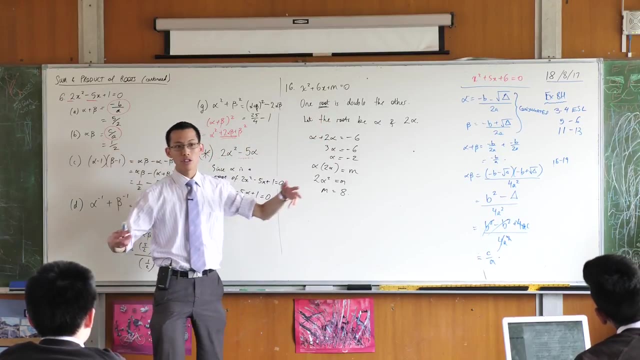 so all we need to do is pop this in and it looks to me like m will be two times four, which you is 8.. Does that make sense? So just define appropriately like so, based on whatever information the question supplies to you, We could have said: one root is one unit away from. 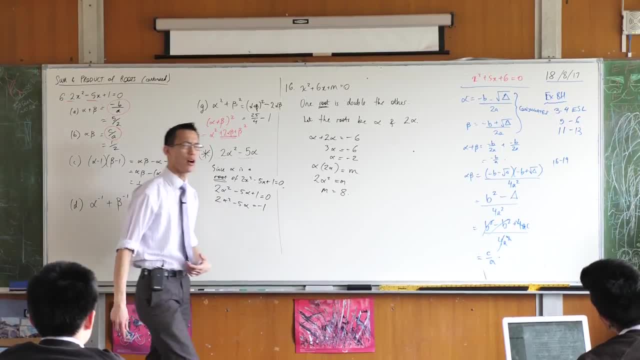 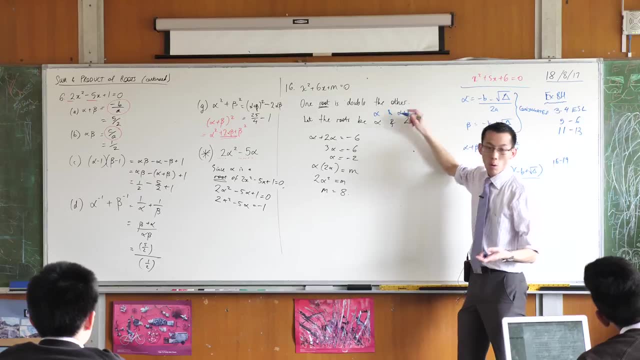 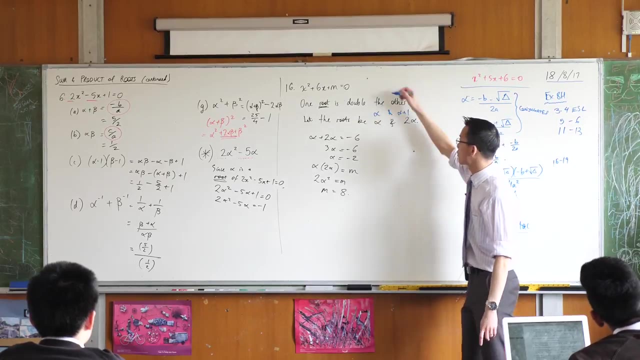 the other root. If one root was one unit away from the other root, then you would define them as alpha and alpha plus 1, or, just as easily, alpha minus 1.. They're still going to be one unit apart. What if one root were the reciprocal of the other? You would define them as alpha and 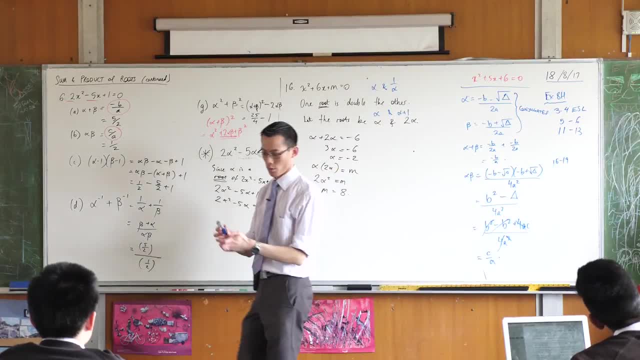 alpha. So you just define them. however, the language of the question tells you to okay.